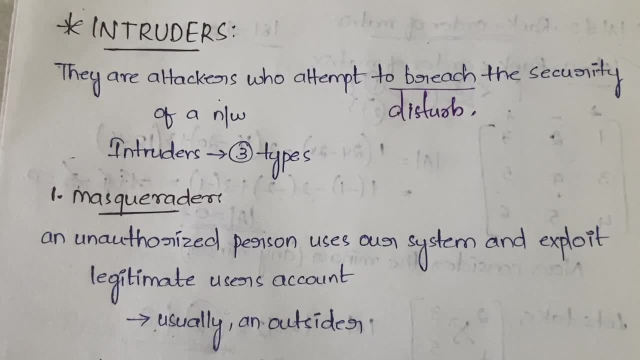 will come, he will use your system and he will exploit the legitimate user's account. so new, new words: exploit and legitimate, so unauthorized means you already know. suppose you are using your phone, you are an authorized person, some x person, some other person is coming and using your phone. 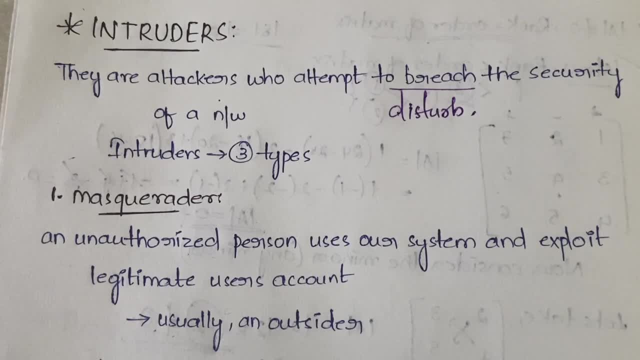 so you don't know. uh, then it is called as an unauthorized person. he is not supposed to use your phone, or he is not supposed to use your atm card, but still he is coming and using. then that is an unauthorized. what do you mean by exploiting and what do you mean by legitimate? legitimate? 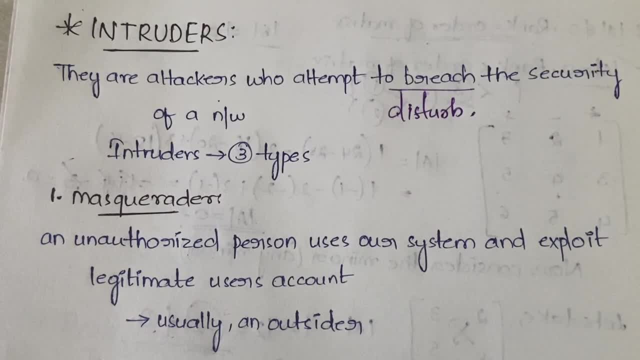 is user is nothing but you. that is the genuine, the original user is the legitimate user. okay, exploit is nothing, but he's going to disturb, he's going to spoil- okay. of course, exploit has a different meaning in traditional english, but in this context, the person that is the Sheila, um, so this is about unauthorized person. that is the unauthorized. 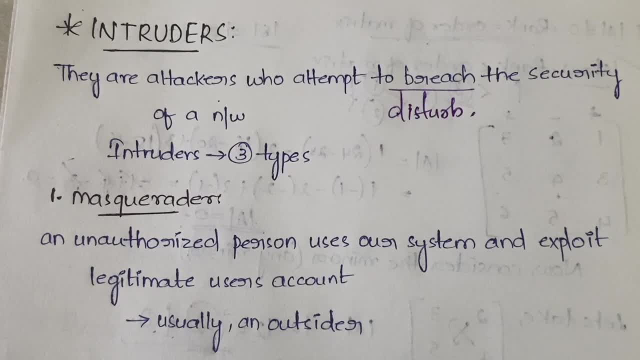 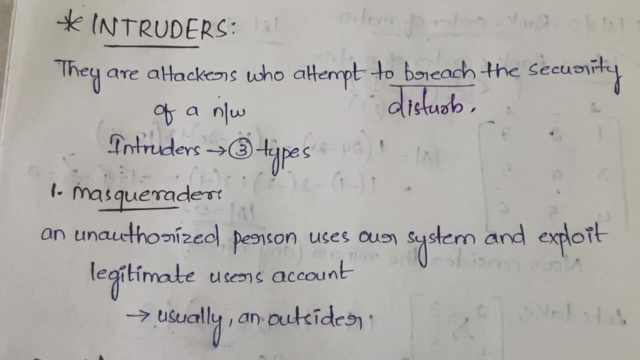 person that is an outsider. some x person will come into our system. he will disturb your system, that is, he will disturb your login, he'll disturb your details. okay, so, that is about the masquerader. usually a masquerader will be an outsider, an outside person. okay so, and the 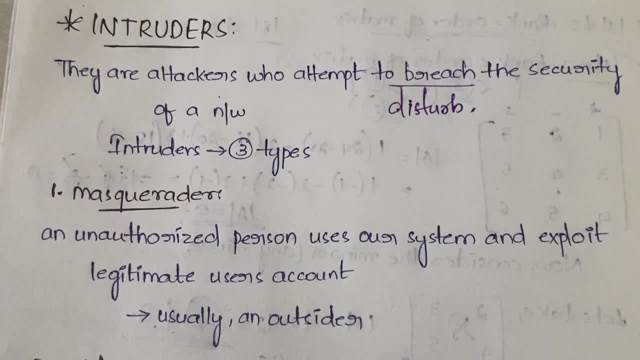 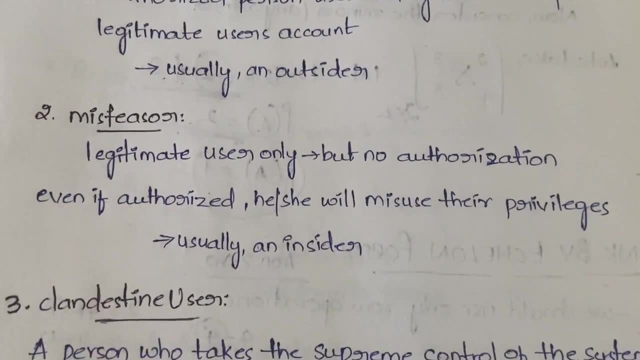 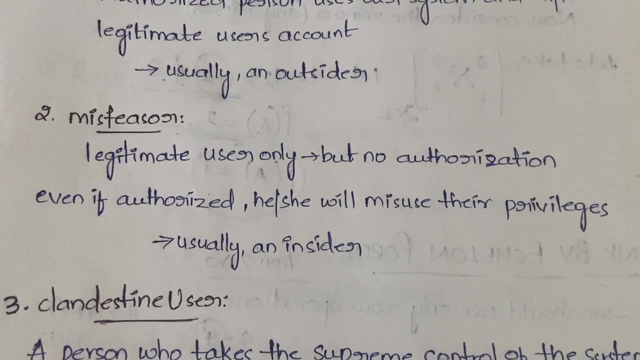 next is a misfeasor. so all the definitions will seem to be same, but at the end you will understand the differences or usage of the system. okay, so the next category is misfeasor. in misfeasor, what will happen is the legitimate user only will have. there will be a legitimate user only, but that user will not have. 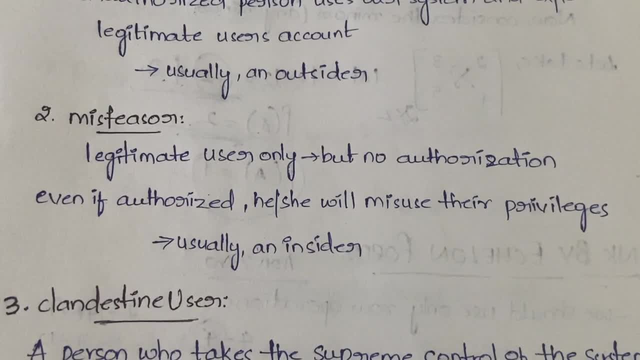 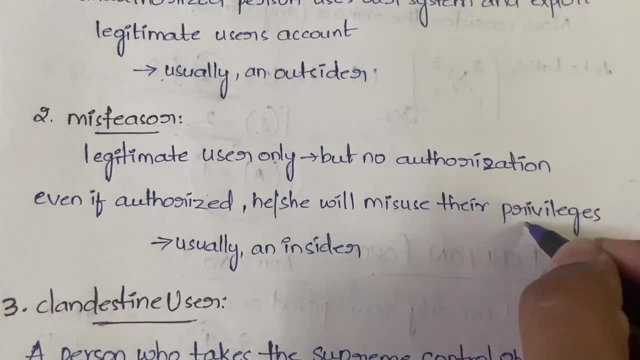 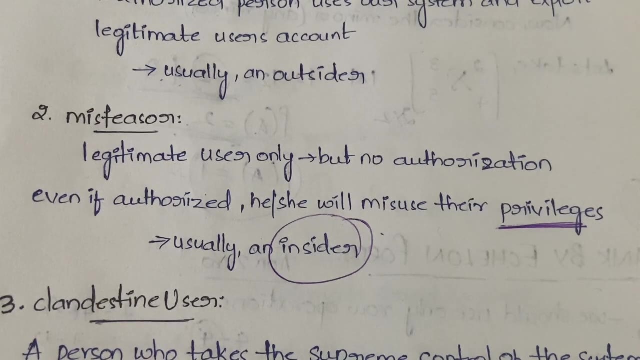 the authorization, he will not have the proper authorization. so, even though if there is authorization, they will use their misuse, their privileges, that is, the permissions. privileges is nothing but permissions they have. okay, usually it is an insider, that is, the person belongs to the organization, that person is a correct person, but still there is no authorization for that. 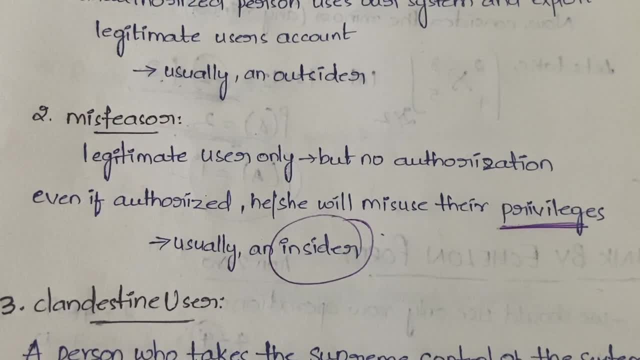 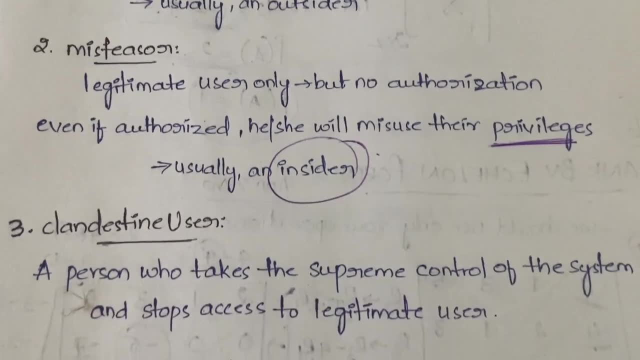 person, even though if it, if the person is having authorization, also, he will not use it properly, he will misuse it or he or she will misuse it. those kind of users are called as misfeasors. next, clandestine user. so in clandestine user. do not take me wrong if i'm pronouncing it wrong. 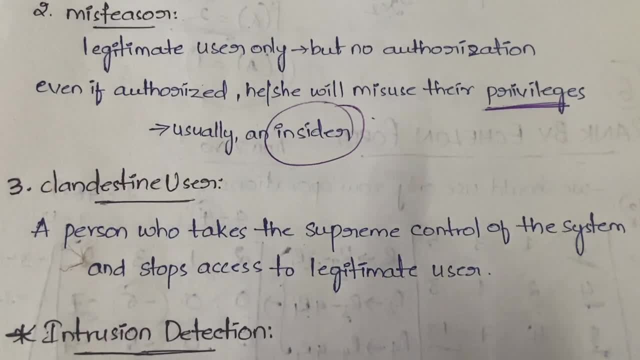 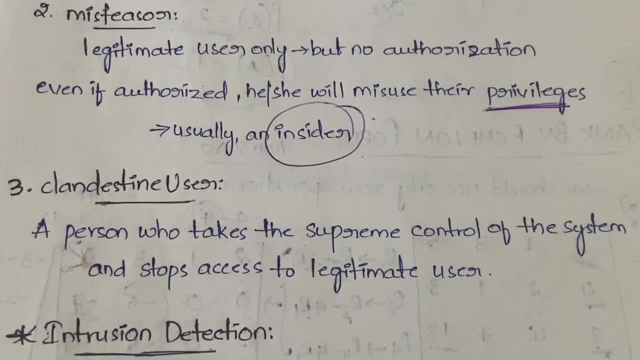 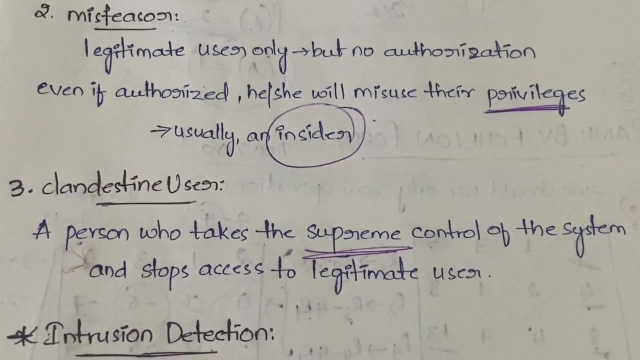 a person who takes the supreme control of the system and stop the access to the legitimate user. that is, some person will come and take control of your computer in such a way that even you cannot use your computer got it, so that is called as a clandestine user. a person will come and he will take the supreme. that is the complete control. 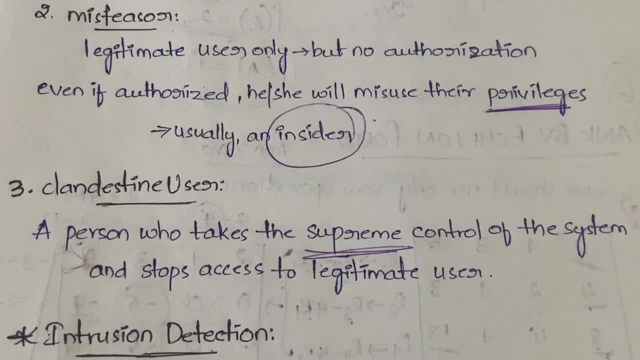 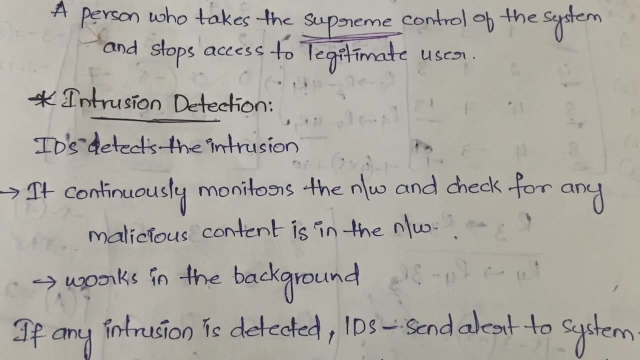 will be taken by that person, so that even you also cannot use the system. okay, this is about the types of intruders. okay, masquerader, misfeasor and clandestine user got it next: intrusion detection. so what do you mean by intrusion detection? intrusion detection is nothing but. 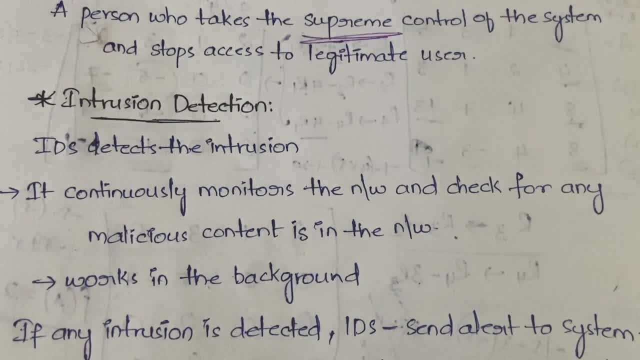 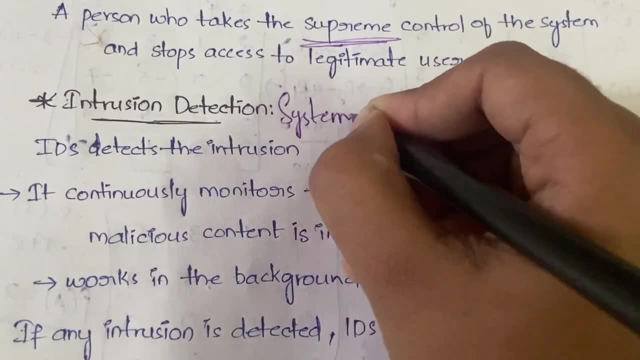 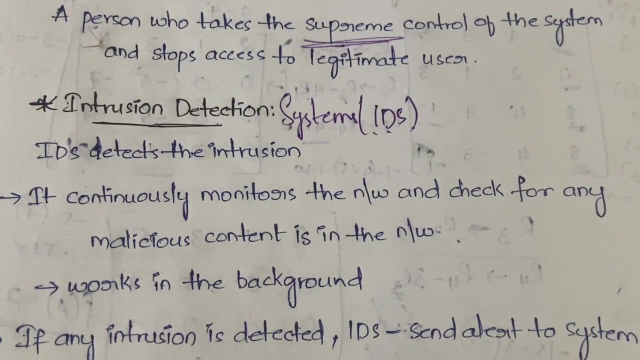 it will identify that the intrusion is happening. okay, so ids is nothing but intrusion detection system. okay, intrusion detection- or you can say intrusion detection systems, also ids, intrusion detection systems. basically they will detect, they will identify the intrusion. so basically what this intrusion detection system, ids, will do is it will continuously monitor the network and check if there are any. if 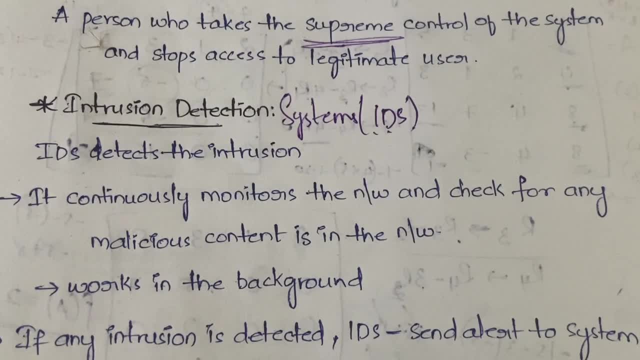 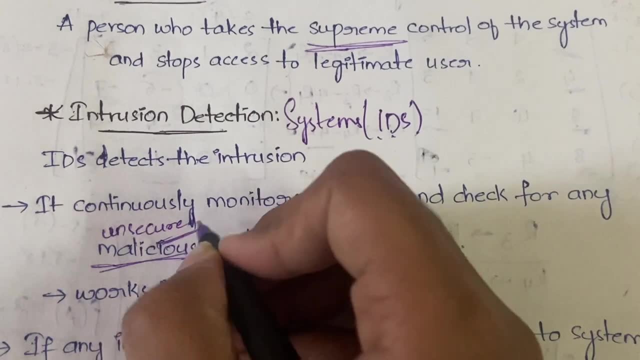 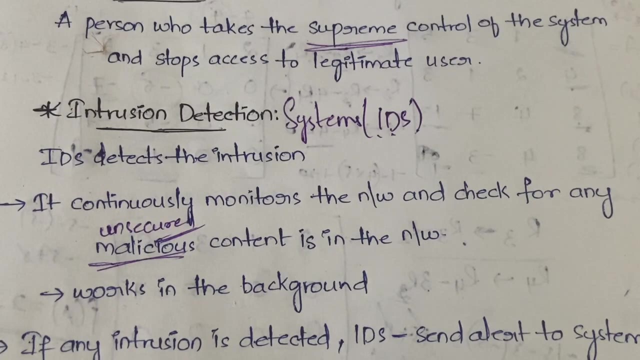 there is any malicious content which is present in the network. malicious content is nothing but unsecured. or you can say you know something which disturbs the security of your system. if there is any unwanted content present in your network or not, it will check the ids, will continuously monitor. 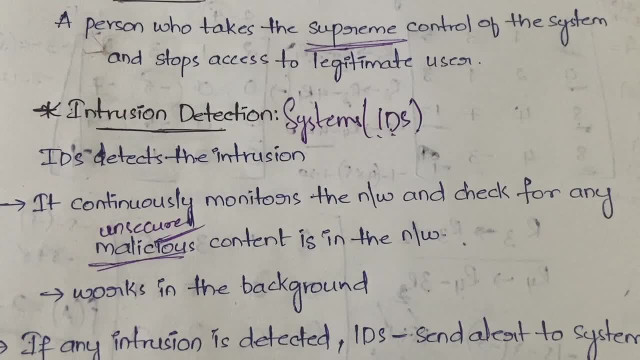 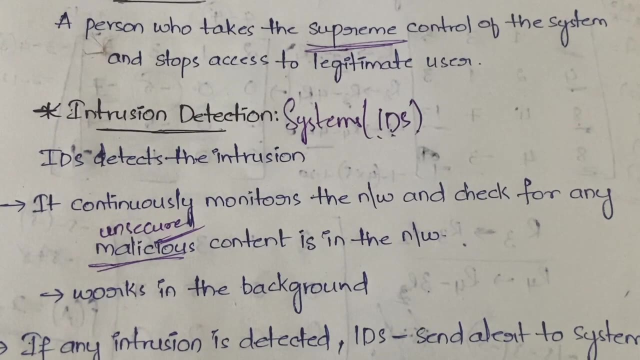 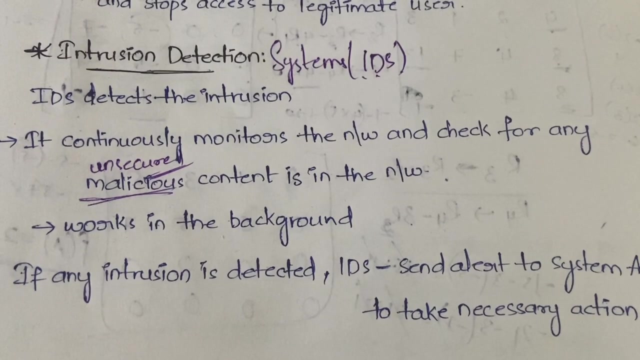 your system will continuously monitor your network. the data packets and all the information that is being transmitted in your system is monitored, and then whatever information it is monitoring, it will check for whether there is any malicious content, or that is, whether there is any unwanted content. check, ok, so it works in the background once if there is any intrusion, detection intrusion. 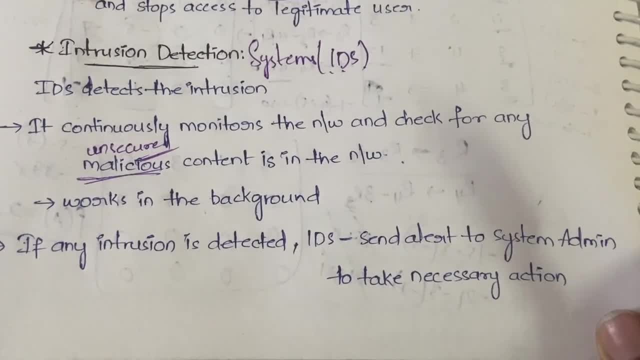 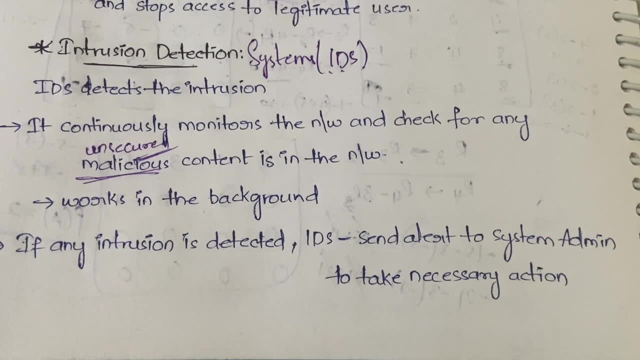 detected, that is, if it identifies any wrong, any unwanted thing is happening, any intrusion is happening in the system, then what the ids will do? it will send an alert to the system administrator saying that an intrusion has happened. an intrusion has been detected. take the necessary action. take the necessary action so that this intrusion will be. what do we? 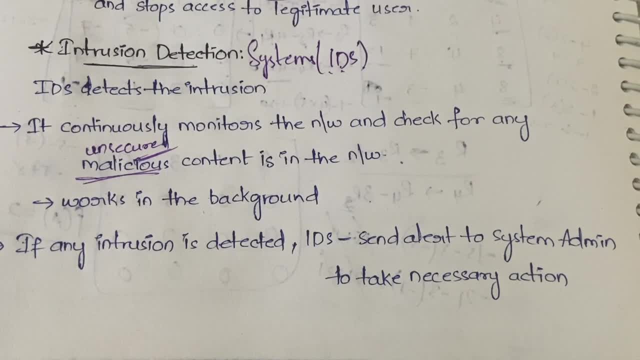 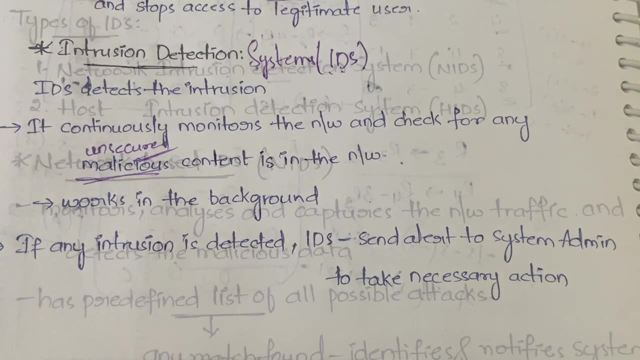 say gone, or it will be corrected like that. ok, so this ids will continuously monitor the network and if any intrusion is detected in between, it will send the notification to the system administrator saying that intrusion has been detected, take the necessary actions in order to rectify it. ok, now coming to the types of ids. we have two types: network based. 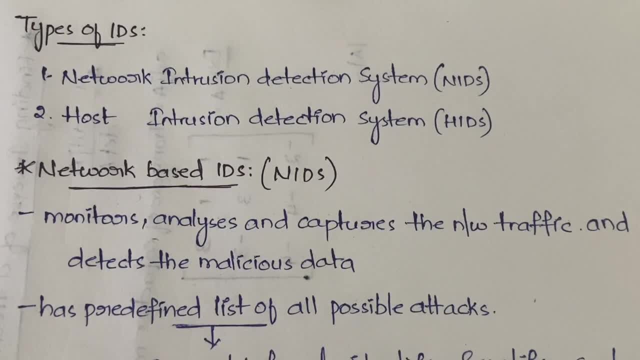 and the host based, network based intrusion detection system- nids in short, and host based intrusion detection system- hids in short. so what this network based will do, what this host will do, we will see. network based ids is nothing, but it works on a particular network, so who are all connected on that particular network? it will work for. 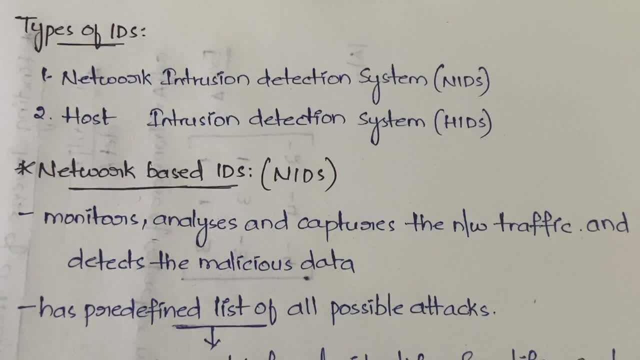 all those devices. suppose in our house we will have a router right. so for that router, if four devices are connected and we implement a network intrusion detection system, then what nids will do? it will perform intrusion detection on all the devices that are connected to that network. ok, 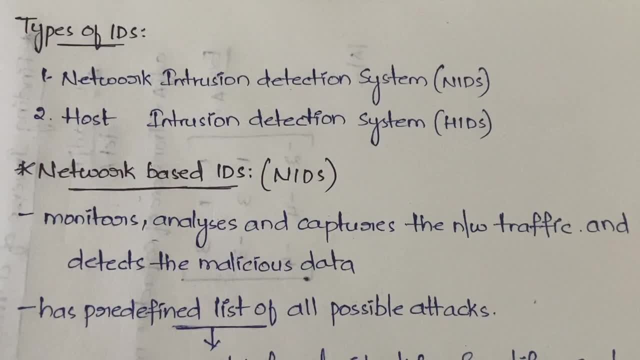 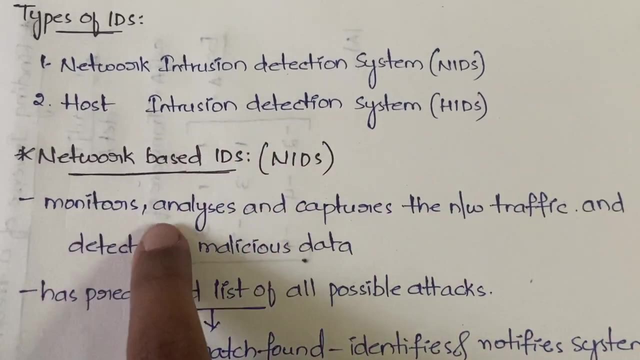 Whereas host is nothing. on a particular host, on your mobile or on your laptop or on your ipad, like that, on a particular host, it will do the intrusion detection. okay, in network what will happen? it will analyze. it is nothing but here ids, nids. it will monitor, analyze and capture the network traffic and detect the. 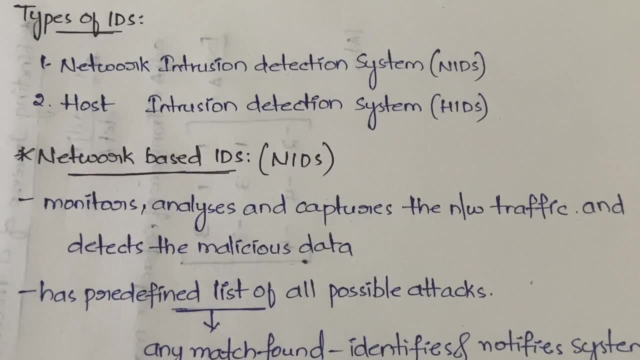 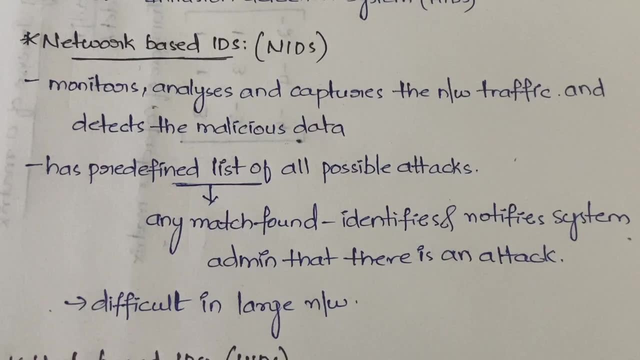 malicious data. again same story, but here what will happen is it will have the list of possible attacks. so what are all the possible attacks that may happen? all those will be in a predefined list, will be there, like how we have predefined data types, predefined functions, predefined libraries. 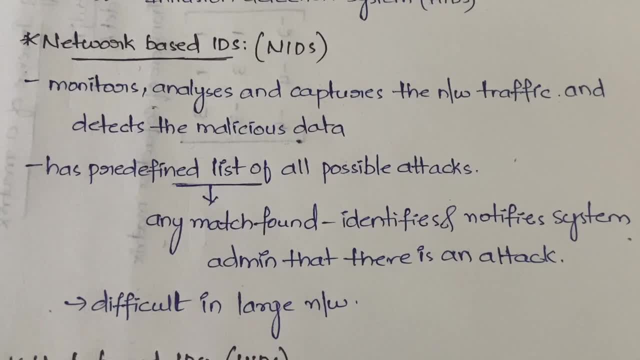 how we have like that some predefined errors or some predefined intrusions will already be stored in the system. okay, so it will check the like with that predefined list. it will check the problems or any intrusions that are being happened. if the if there is a match. if the match is found, then it will send a notification or an alert to. 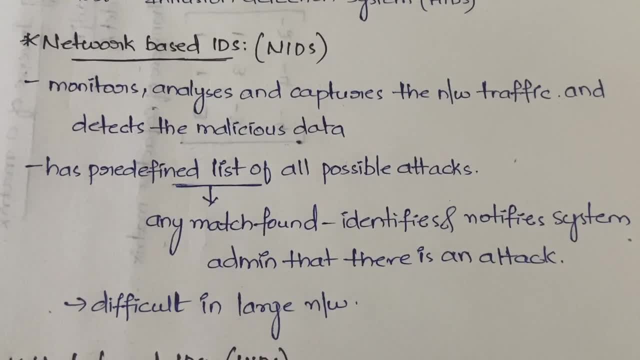 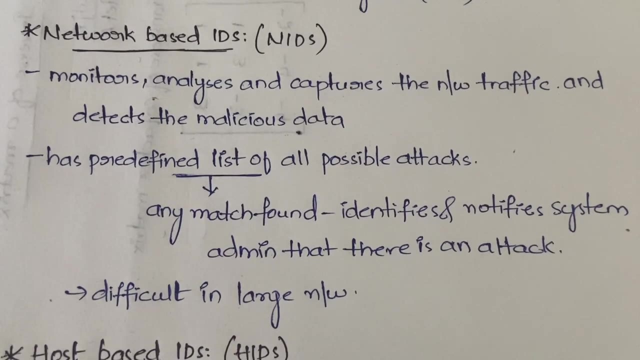 the system administrator saying that there is an attack. okay, so this is what happens in case of nids. nids will have a predefined list, right, it will compare along with that against that list and give the notification if there is any error done. next, it is difficult in large network. 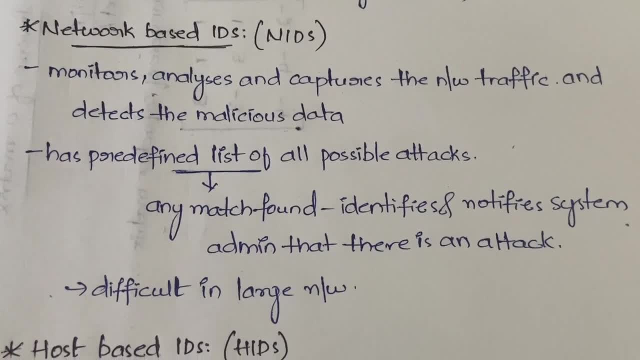 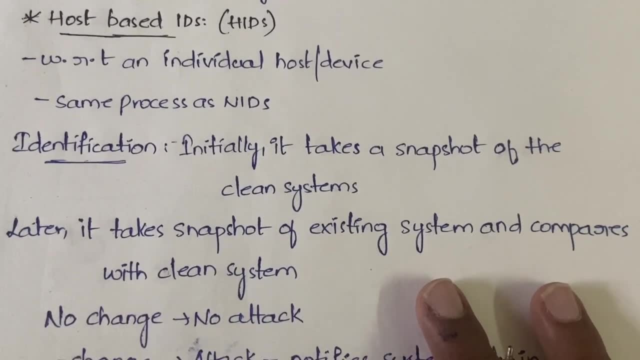 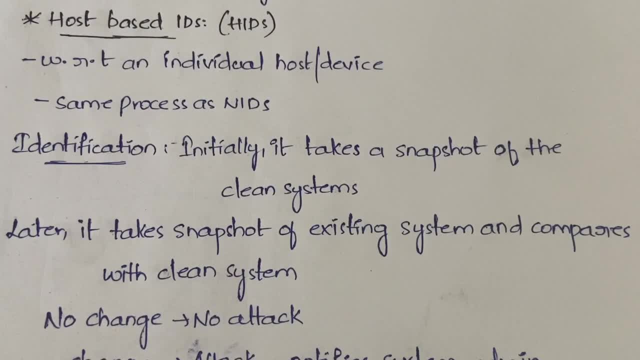 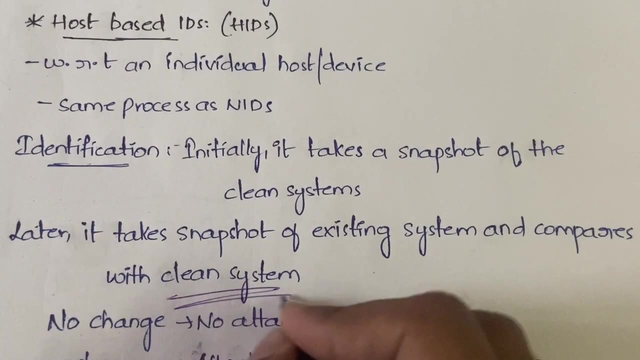 will do the same process, that is, it will monitor, analyze and captures and it will detect, it will match all that. but here, how? there there is a list of errors, but here what will happen is initially clean system that is, clean system is nothing but a system with no errors. 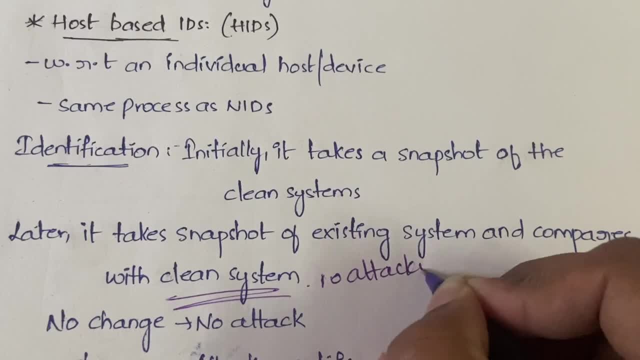 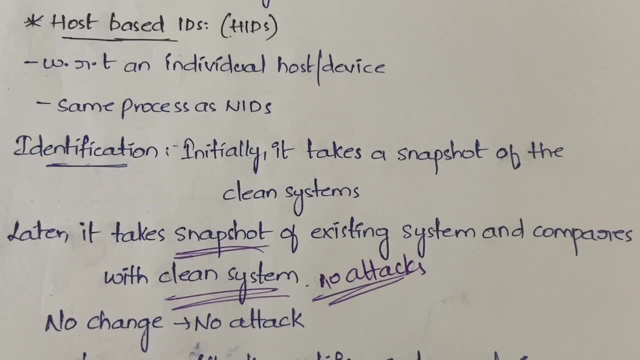 with no defects or no attacks. we can say a system which is having no attacks. so in that system snapshot is taken. snapshot is nothing but screenshot. you take the picture of that system. okay, if it is clean, if it is having no errors, then how the system looks like. 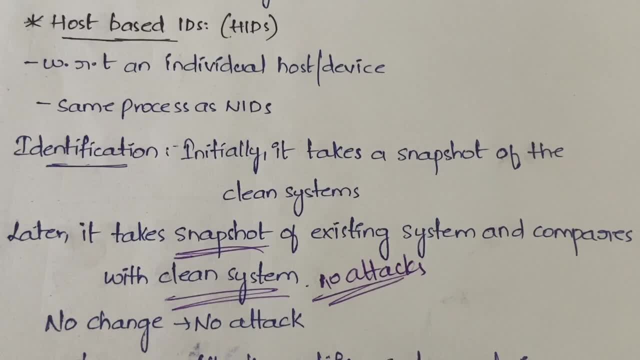 system in the sense it could be an application, or it could be a screen of your laptop or it could be a website, anything so initially, before any errors or before any attacks, how the screen looks, it will take the picture of it now. later on it keeps on comparing with that. 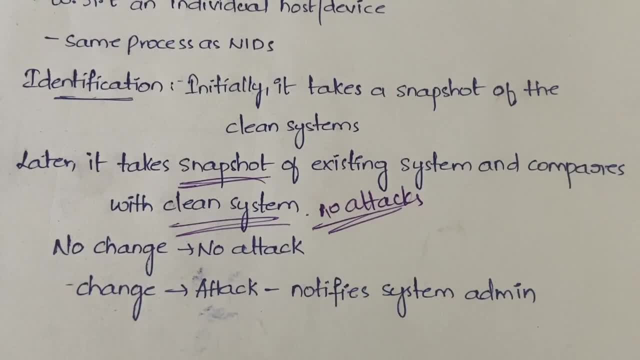 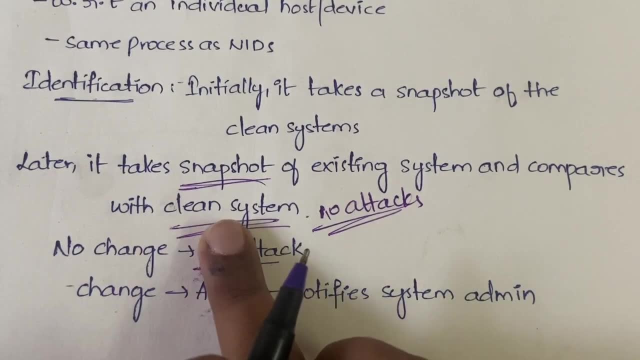 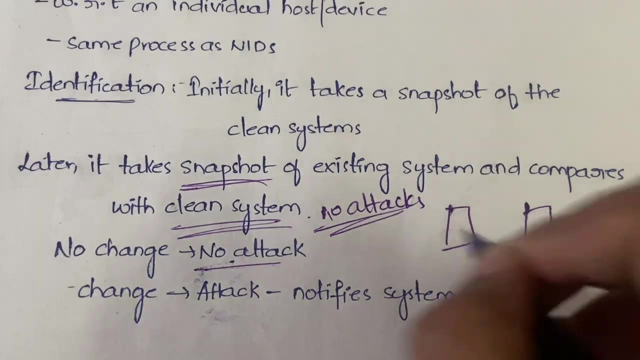 snapshot which has been taken. okay, if there is no change, then we say that there is no attack. okay, so the snapshot which we have taken, the snapshot of the clean system and the snapshot of the present system is matching. then we say that there is no attack, suppose, if it. 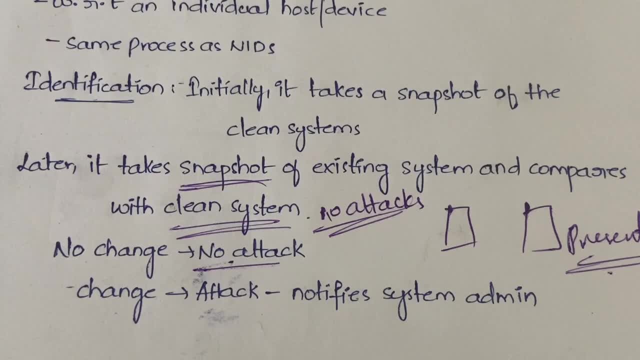 is not matching if there is any change in the system, like the color or the you know anything. if there is any change, then we identify that some attack has been happened and that notification will be sent to the system administrator and the system administrator will be taking the necessary actions that 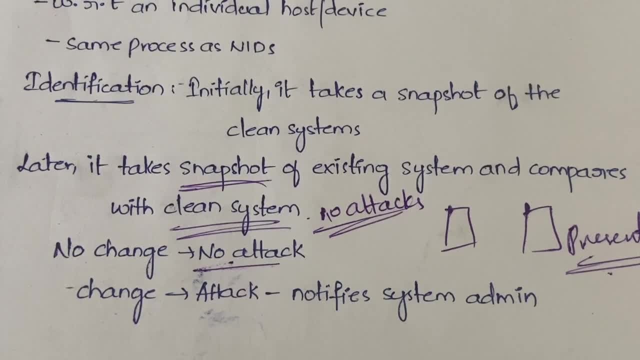 is blocking those people or, you know, changing the address or changing the password or whatever necessary actions will be taken by the system administrator. okay, this is what happens in host based intrusion detection system. both same: it will identify the intrusion and it will send the notification to the system administrator. but the difference between network and host is network. 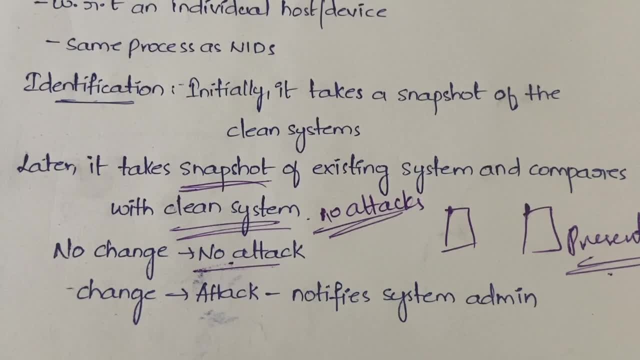 it operates on the complete network. there is host operates on a particular device and in network based, what will happen? it is compared with a predefined list. in case of host based, what's happening? it is compared with the snapshot of the clean system. that is the difference between two. 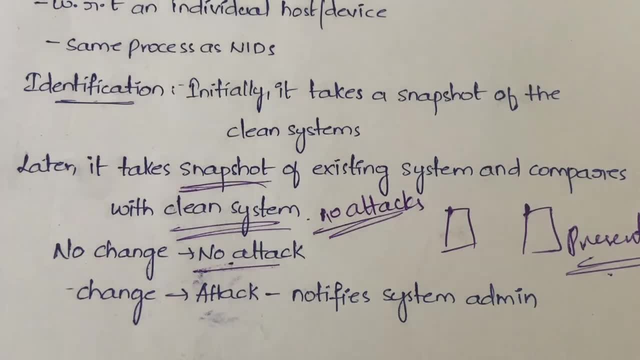 got it. so that's all for this video. thanks for watching the video till the end. if you're still having any doubts, let me know in the comment section. i'll definitely try to clear all your doubts. for sure, let's meet up in the next coming video with another topic. till then, stay tuned to.